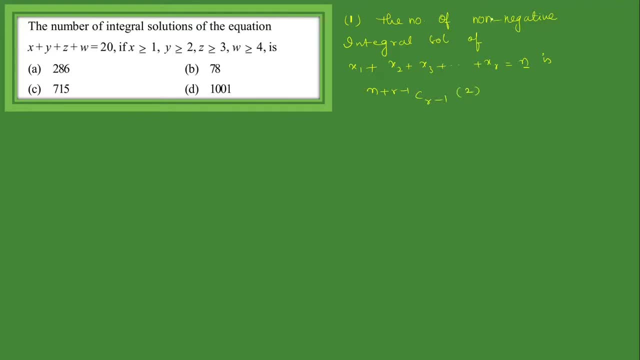 have seen this. And the second rule: instead of the number of non-negative integral solutions, number of positive integral solutions for the same equation. for the same equation, how many positive integral solutions are there? What is the rule? we have n minus 1, c, r minus 1.. 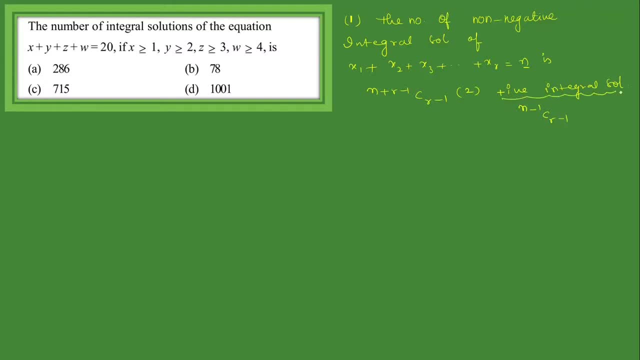 For the same equation. if you want number of positive integral solutions, we have the formula n minus 1, c r minus 1.. And if you want only non-negative integral solutions, that is x 1 plus x 2 plus up to so on. x r is equal to n equation. the answer is n plus r minus 1, c r minus 1.. 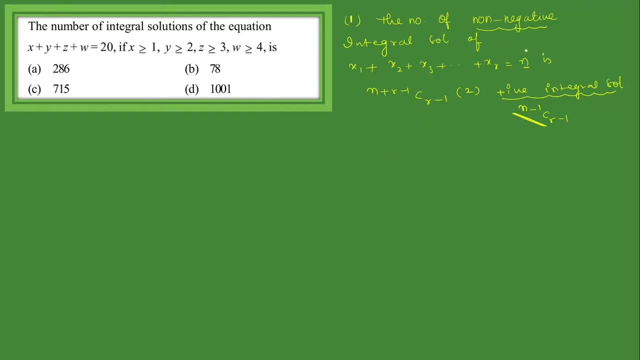 This is nothing But the number of ways of distributing n identical objects into r distinct boxes. so that no restriction, without any restriction, without any restriction. if you want to distribute n identical object into r boxes, the direct result, you can use n plus r minus 1, c r minus 1.. 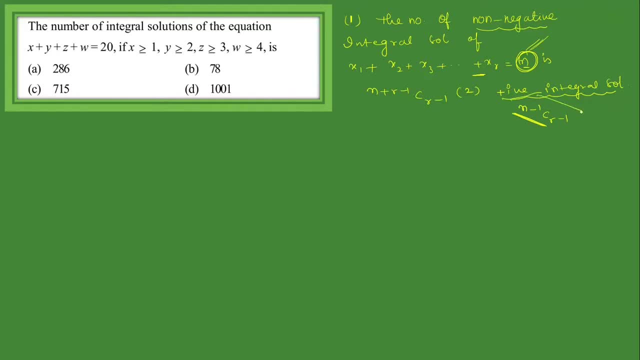 Whenever no box empty means at least one object should be there in the box. then n minus 1, c, r minus 1.. So this is the. these are the two properties, these are the two rules we have seen in the previous two lessons. right Now, here we are going to apply. 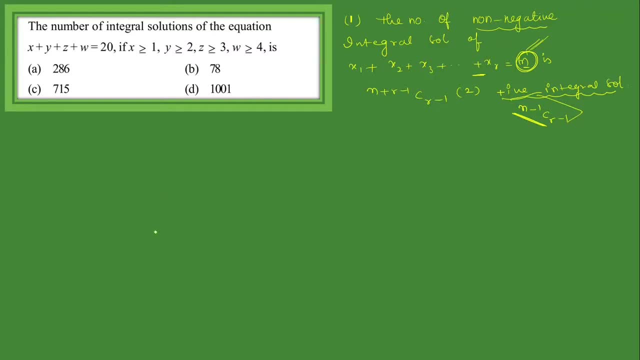 how to apply these rules into different situations. okay, So we will solve three to four problems in this class today. Now here, the first problem is: we have to find out the number of integral solutions of this equation satisfying some condition. Can you see the equation? What is? 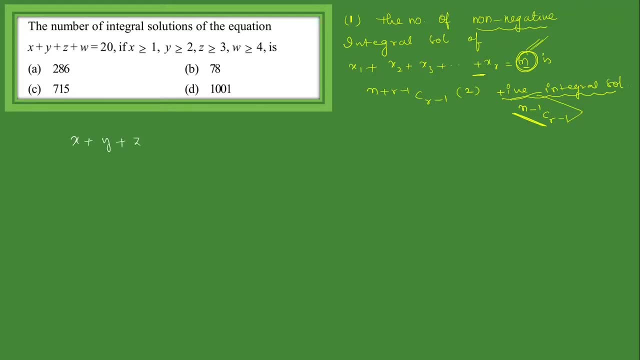 equation given to us: x plus y plus z plus w, w is equals to 20. for this equation, right Say equation number one- For this equation you have to find out integral solutions. He did not mention whether it is a non-negative. 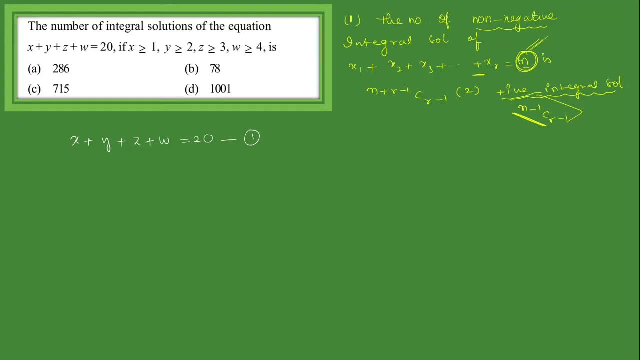 integral solutions or positive integral solution. But it is mentioned clearly that x is greater than r equal to 1, and y is greater than r equal to 2, and z is greater than r equal to 3 and w is greater than r, equal to 4.. So, satisfying these conditions, x is greater. 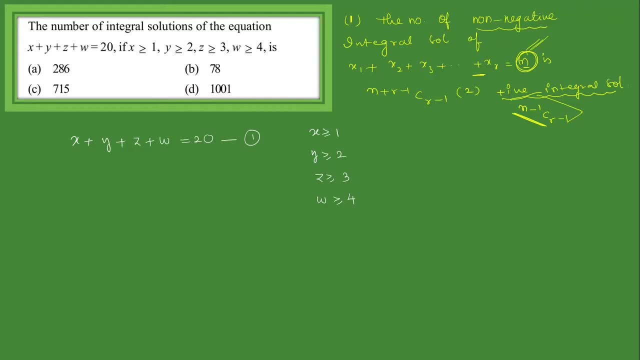 than or equal to 1, y is greater than or equal to 2, and z is greater than or equal to 3, and w is greater than or equal to 4.. How many solutions are there for this equation? Now, what we are going to do: we are going to convert this equation into the situation 1 or 2, which 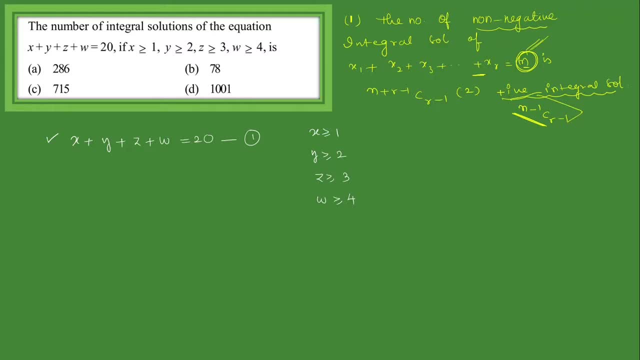 one we are going to do is first one. Now, what I am going to do, you see here, because of x is greater than or equal to 1, from this what you can say, x minus 1 is greater than or equal to 0- means x minus 1 is non-negative. Similarly, y is greater than or equal to 2. 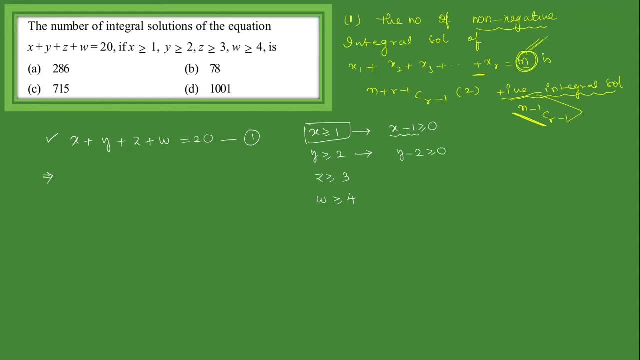 means y minus 2 is greater than or equal to 0, means y minus 2 is non-negative. So z is greater than or equal to 3 implies z minus 3 greater than or equal to 0,. w is greater than or equal to 4 implies w minus 4 is greater than or equal to 0. So therefore this x. 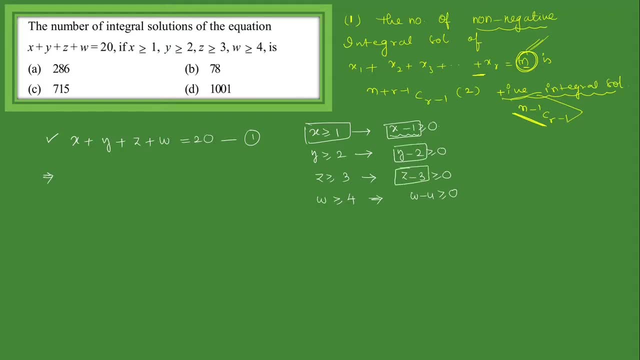 minus 1, y minus 2, z minus 3, w minus 4.. Now, these four values are what? Non-negative negative? These four values are non-negative. Is it clear? So now, whenever you have non-negative, 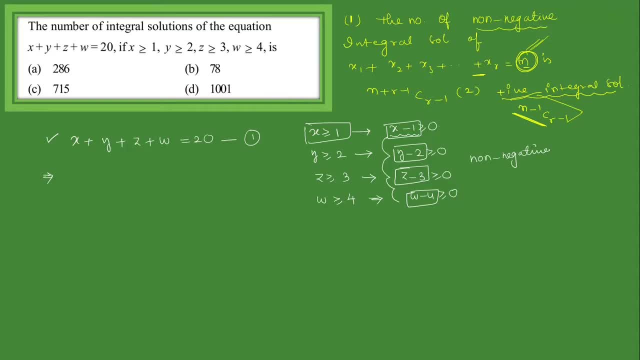 variables. in your equation you have a direct formula to find out non-negative integral solution. What is that? n plus r minus 1, c, r minus 1.. Here n is right-hand side number, r is number of variables or number of boxes. Now what I am going to do? I am going to change. 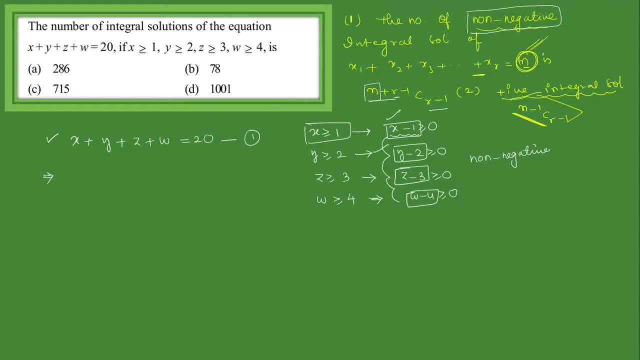 this equation, in which we will see this: x minus 1, y minus 2, z minus 3 and w minus 4.. How can you make it So? from x, what you do, You subtract 1.. From y, what you do You. 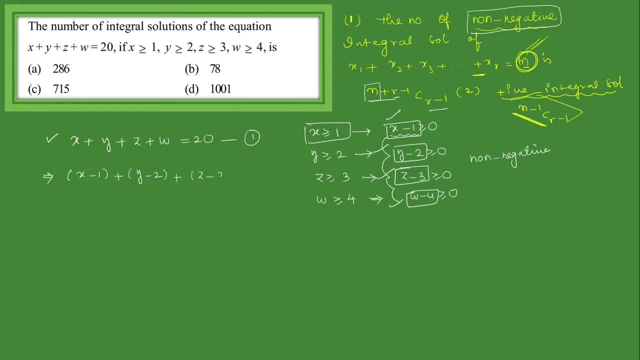 subtract 2.. Again from z, you subtract 3, and again from w, you subtract 4.. So you have subtracted how much? 1, 2, 3,, 3,, 6,, 4, 10.. So that 10 we subtract from the right-hand. 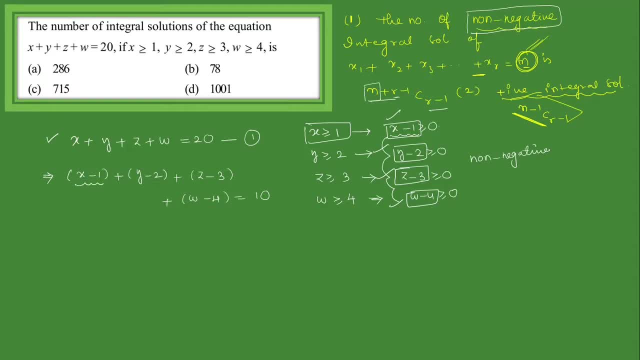 side. Now, instead of x minus 1, for some time I will say it is capital X, and for y minus 2, I will say it is capital Y, and for z minus 3, I will say it is capital Z, and this is capital W, which is equal to 10.. Now you got a different. 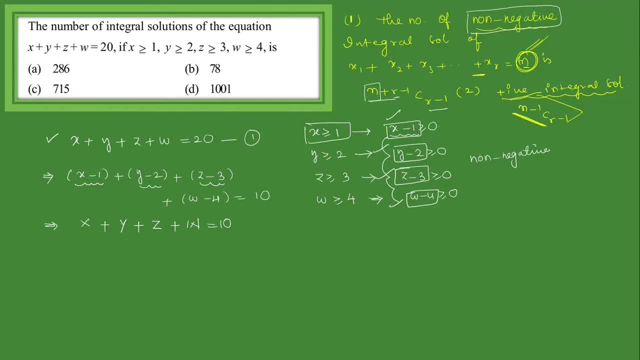 equation. Little bit conversion is done here. The same equation is converted into the another form, where this capital X, capital Y, capital Z, capital W- You can see this is I suppose it as capital X, this one I suppose it as capital Y, and this z minus 3, we suppose it. 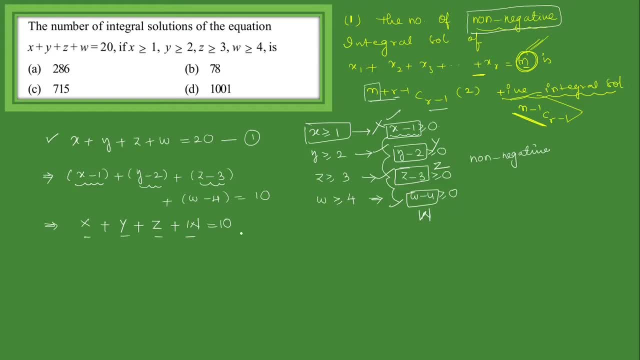 as capital Z and this is capital W. but you can see here X is greater than or equal to 0, y is greater than or equal to 0, and z is greater than or equal to 0 and w is also greater than or equal to 0.. So what are the variables you are seeing in the equation capital X? 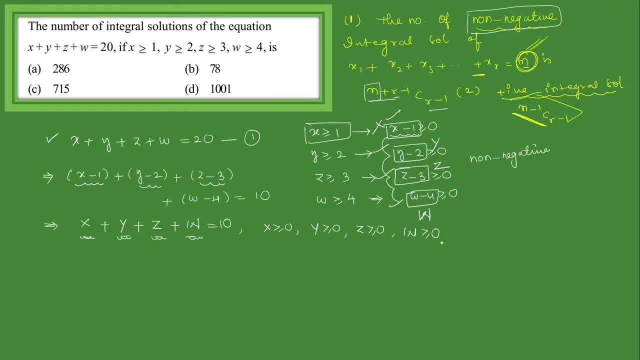 capital Y, capital Z, capital W. these all are non-negative. So, indirectly, what you are going to find is the number of the number of integral solutions of 1, the number of number of integral solutions of 1, satisfying these conditions: x. greater than or equal. 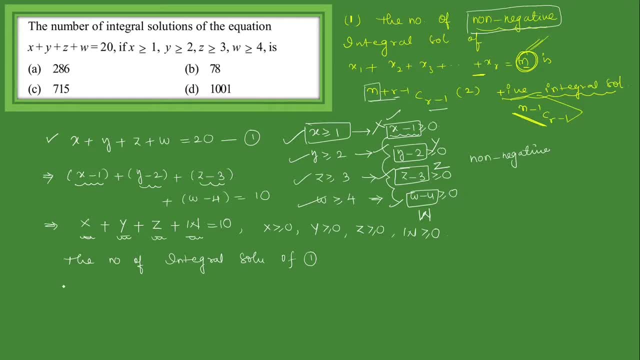 to 1, y greater than or equal to 2, z greater than or equal to 3, w greater than or equal to 4, is same as the number of solutions, the number of non-negative integral solutions. I can say why. I can say because we made it like that, x greater than or equal to 0,. 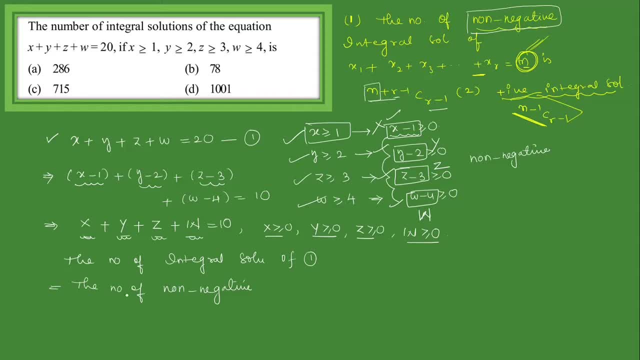 y greater than or equal to 0, z greater than or equal to 0, w greater than or equal to 0.. So we want the number of non-negative integral solutions, integral solutions of the equation which is converted. this one say: this is number 2.. So number of non-negative. 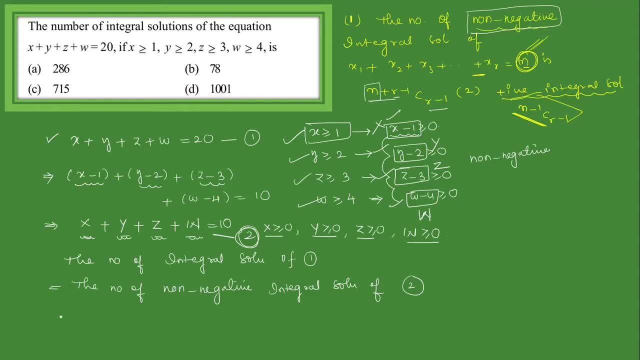 integral solutions of 2, you have to find out. So this is equals to what Number of non-negative integral solution formula is n plus r minus 1, c r minus 1.. In this n is number of identical objects. this is number of identical objects. you can say, or it is: 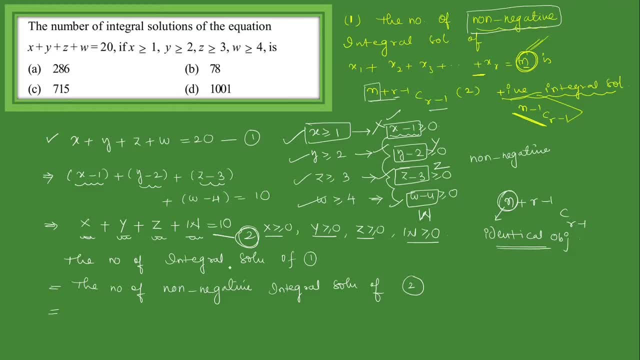 a right side number in your equation. So in the equation, what is the right side number here? 10.. So n value is 10 and what is r Number of different boxes or number of variables involved in the equation? How many variables involved in the equation: x, y, z, w, 4 variables. 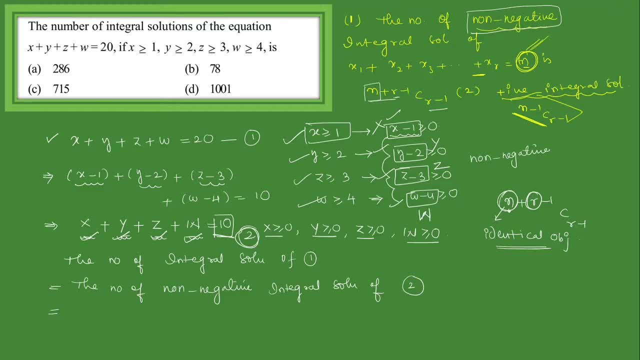 So r value is 4 and n value is how much 10.. So the answer is 10 plus 4 minus 1, c, 4 minus 1, which is 13c3.. Now, if you want, 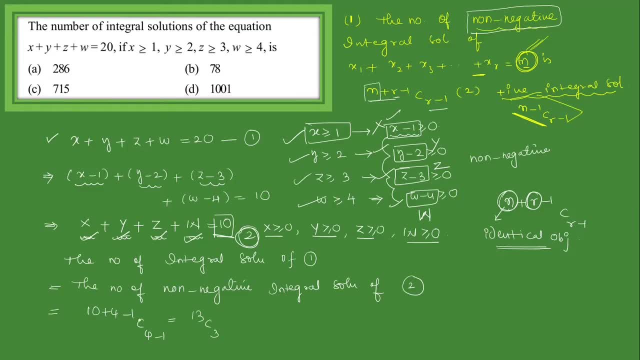 you can calculate this: 13c3, 10 plus 4, 14 minus 1, 13c3.. So you can calculate, if you want 13, into what is that? 12 into 11 by 3 into 2 into 1, 6,. so 6, 2 is a 12.. So 13. 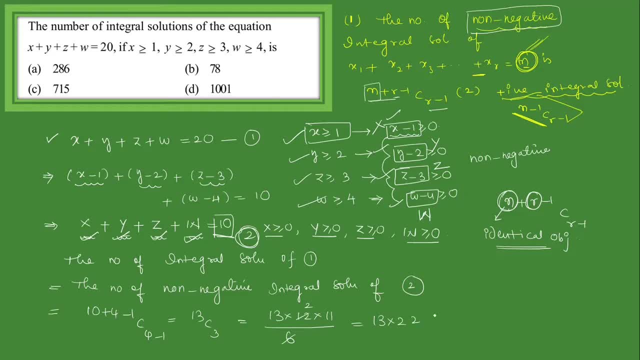 into 22,. if we calculate this, 13,: 2 is a 260 plus 20.. 386 minus 22 is a 286, which is 286.. So 13 into 22, which is 286, you can see which is. 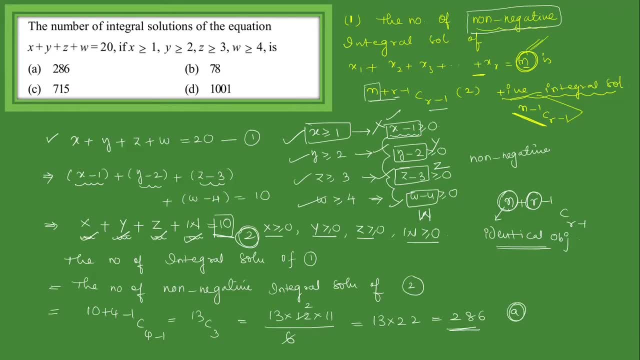 there in the A option. So this is the way of applying the rules. what we learned in the previous two lessons- number of non-negative integral solutions and number of positive integral solutions. So here in this question he is not asking number of non-negative integral solutions. 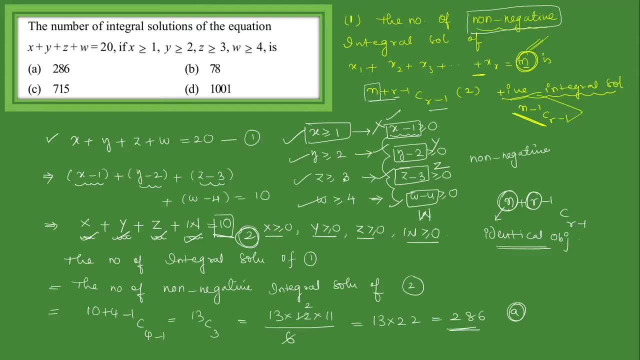 something given: x is greater than or equal to 1, y is greater than or equal to 2, z is greater than or equal to 3, w is greater than or equal to 4.. So we have dreamt of please. 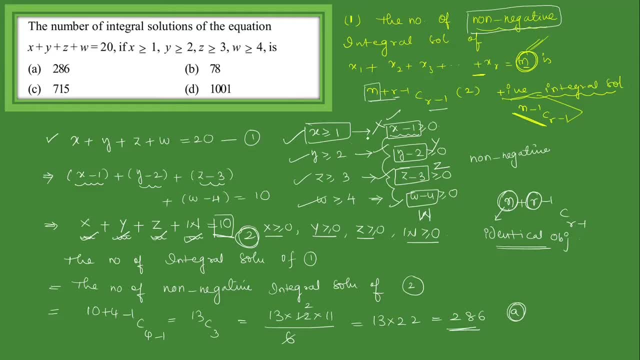 write a little journal for this. So in this question our goal with written measurements is to put whatever equation is pointed out to the answer off the paper. Theuttering solution, but using here x minus 1 and y minus 2 and z minus 3 and w minus 4, we converted the given. 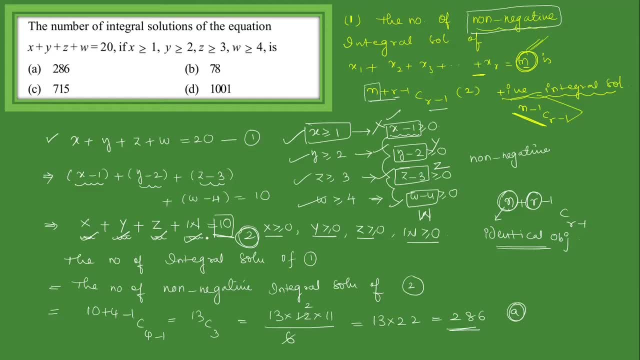 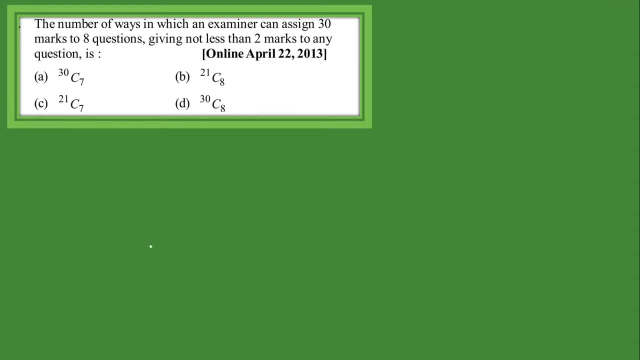 equation so that the variables are non-negative. right, so that we can use the first property. now let's see one more question. now this is question from 2013, online, april 22, based on the same concept. now we can check this: the number of ways in which an examiner can assign 30 marks to. 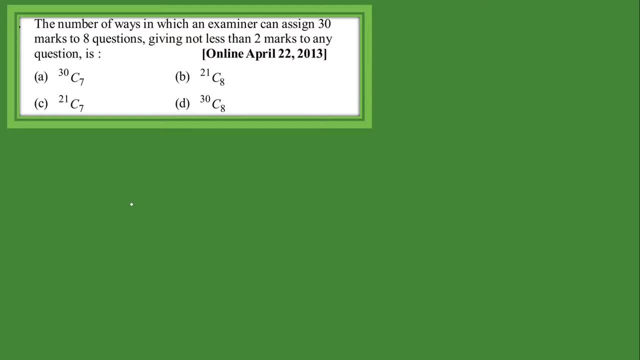 eight questions, right, giving not less than two marks to any question. so total number of questions: how many? total number of questions we have eight and how many marks we have to assign to these eight questions. so in total, we have to assign 30 marks to these eight questions. right, but you should. 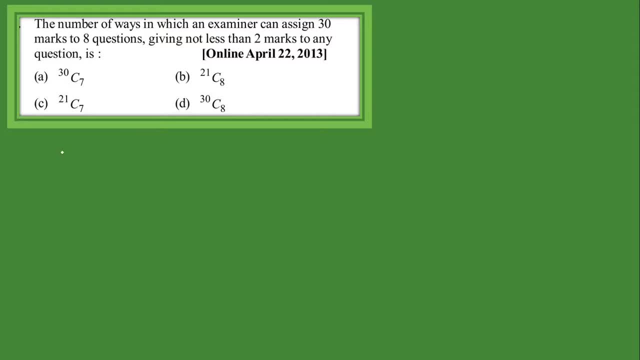 not give less than two marks to each question. so here we have question number one, question number two, question number three, question number four, right, so like question number three. question number four, right, so like question number three. question number four, right, so like Question number 5, and question number 6 and question number 7 and question number 8.. 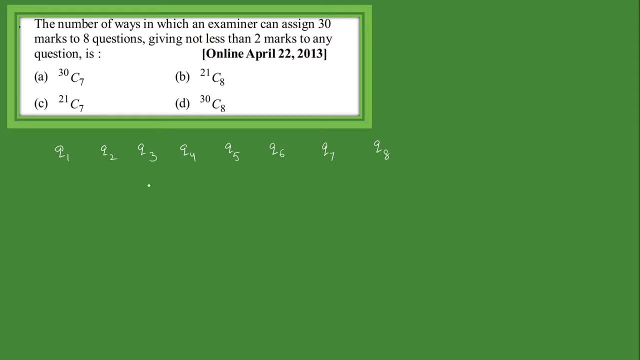 So totally you have 8 questions. We have to assign some marks to Q1 and some marks to Q2 and then some marks to Q3.. Like, for example, you can assign 3 marks to the question 1, 2 marks to the question 2.. 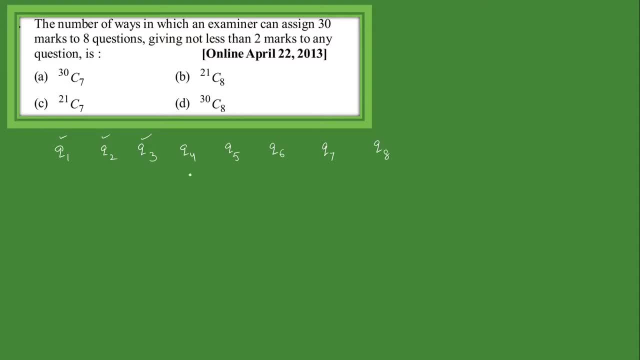 For example, you can give some 3 marks to question 3.. Like this, you have to assign marks to each question randomly, But what is the condition Then? each and every question must be assigned, must be given at least 2 marks. 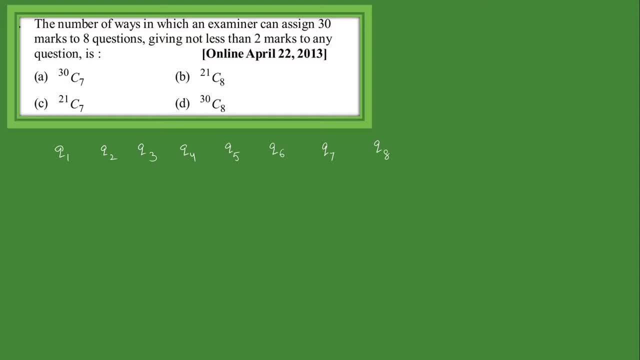 2 marks are more than 2 marks. You cannot give 1 mark or 0 marks to a question. Minimum marks should be given to each question is 2 marks. But after giving that marks, if you add all those marks- Q1 plus Q2 plus Q3 plus Q4 plus Q5 plus up to so on- Q8 should be how much. 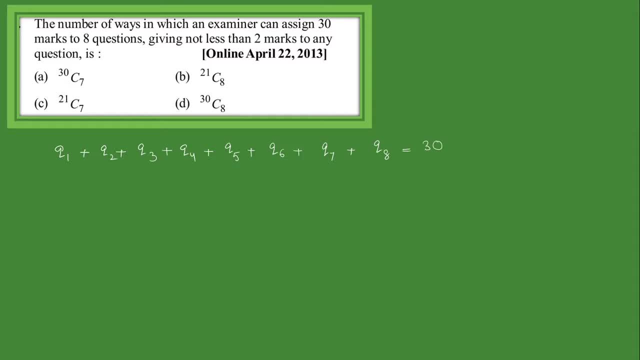 30 marks, Yes or no? So here you got an equation, Invitational So, in which you have 8 variables and you know each QI. what is that? Each QI is greater than or equal to 2.. 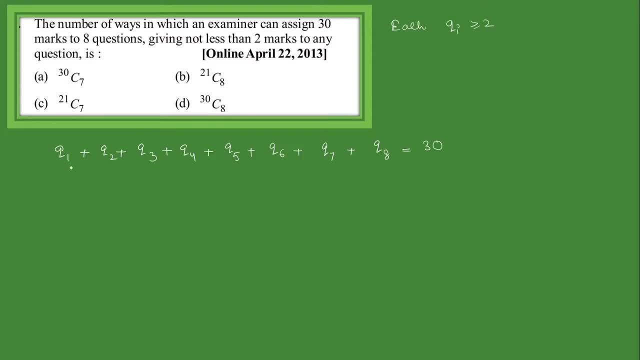 What is the meaning of this? Whatever the marks we have given to the first question, it should be greater than or equal to 2.. Whatever the marks you are allotting to the second question, it should be greater than or equal to 2.. 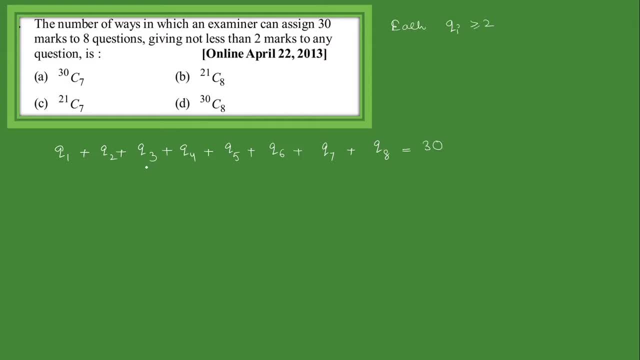 Like that, each and every question. for each and every question, the minimum number of marks is 2.. So, therefore, QI is greater than or equal to 2.. What does it mean? Q1 is greater than or equal to 2.. 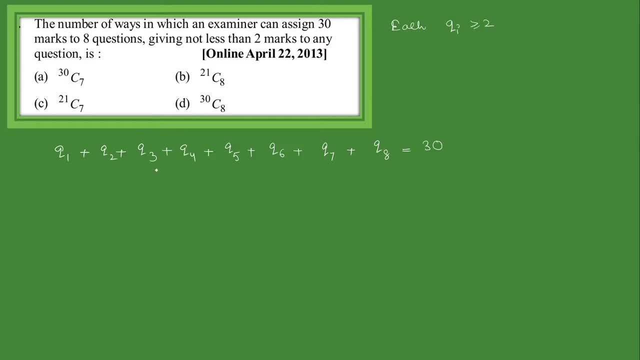 Q2 is greater than or equal to 2.. Q3 is greater than or equal to 2.. Likewise, each QI is greater than or equal to 2 implies what you can do here. QI minus 2 is greater than or equal to 0.. 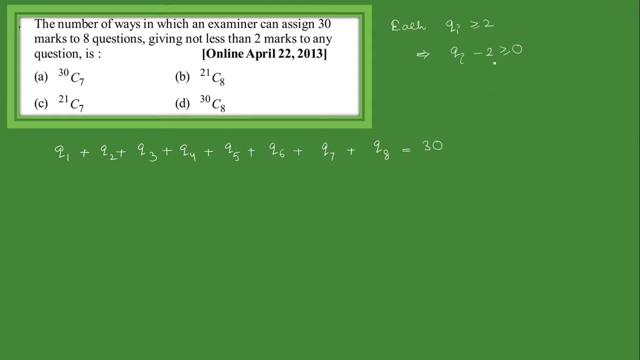 Yes or no. QI minus 2 is greater than or equal to 0.. What does that mean? What does it mean? Q1 minus 2 is greater than or equal to 0.. And also, Q2 minus 2 is greater than or equal to 0.. 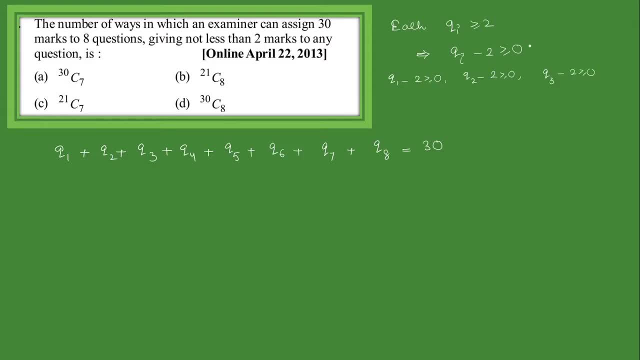 Q3 minus 2 is greater than or equal to 0. So this is true for all. I is equal to 1, 2.. So q1 minus 2 is non-negative. q2 minus 2 is non-negative. q3 minus 2 is non-negative. 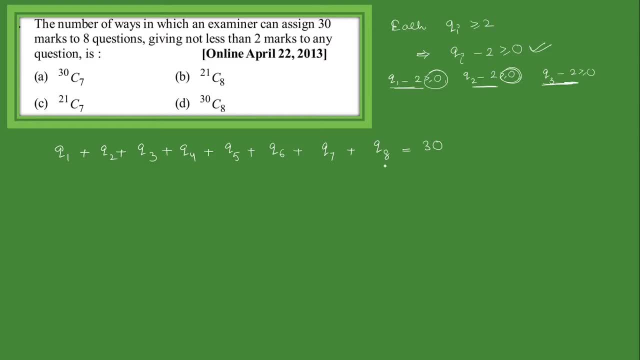 So you can use that non-negative concept from the previous problem, right? So what I am going to do, Can you guess? I am going to subtract 2 from q1.. Similarly, I am going to subtract 2 from q2 and 2 from q3.. 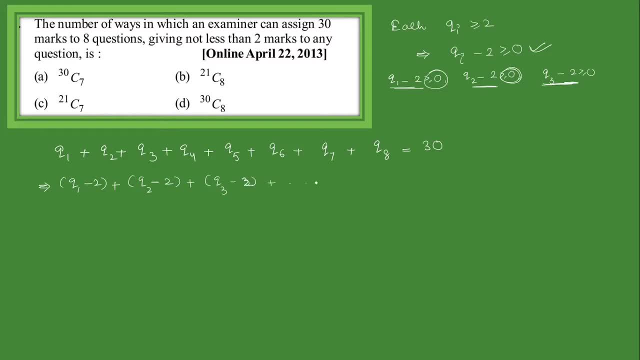 So I will continue this up to q8.. From q8 also, I am going to subtract 2.. So totally, how many 2s? we subtracted from the left-hand side? Two 8s, 16.. So you have to subtract that 16 from the right-hand side also. 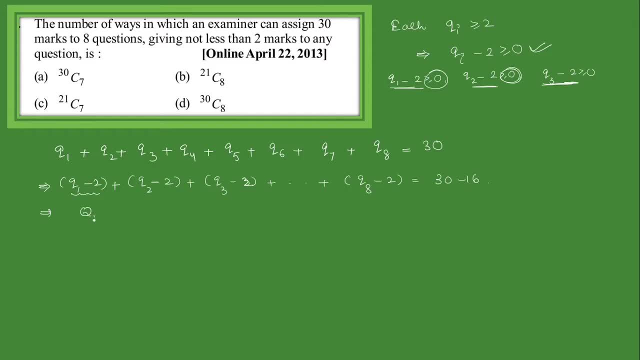 So now I will suppose this q1 minus 2 as capital Q1,. let us say: Is it good, Capital Q1, or this is capital Q2 and capital Q3, plus up to so on capital Q8.. Capital Q8, which we have 14.. 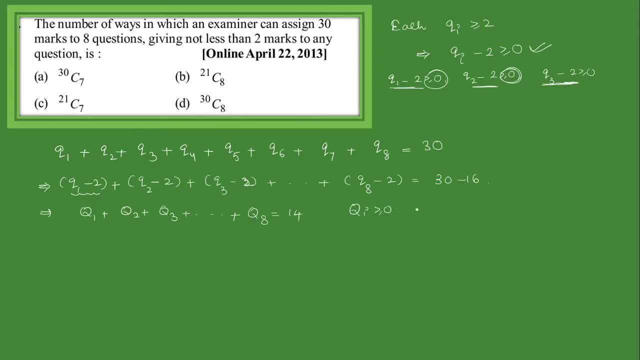 Now here, each qi is greater than or equal to 0, means each and every number in this equation, variable in this equation, is non-negative. So what you have to find out here, You have to find out the number of non-negative. 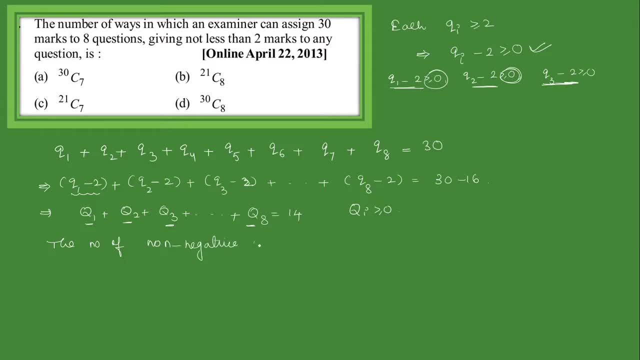 you have to find out the number of non-negative integral solutions, number of non-negative integral solutions of this equation, of the equation just now we have applied, We have obtained. So what is the formula for number of non-negative integral solutions? Once again, I repeat: n plus r minus 1, c r minus 1.. 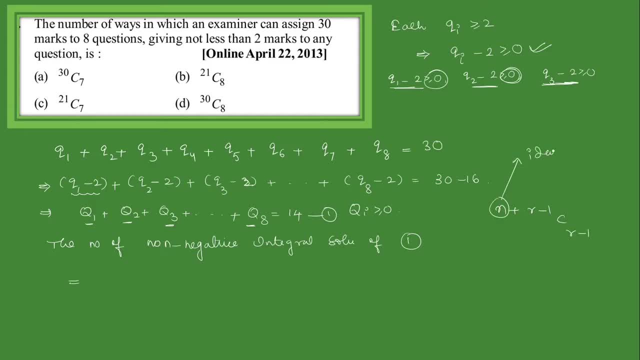 What is n here? n is identical objects. How many identical objects are there? Or RHS number. What is the number you are seeing in the RHS of the equation? And what is r? r is number of boxes. You can say number of boxes. 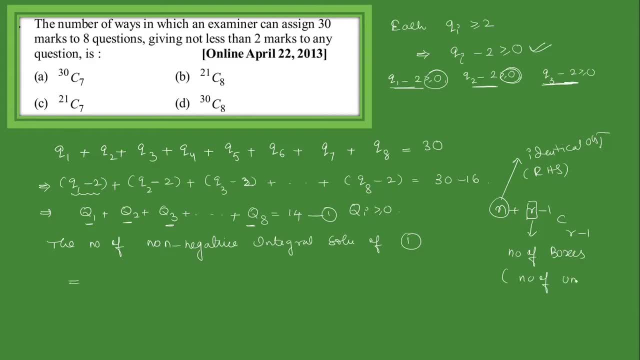 Or if you see in the equation number of unknowns or number of variables. Now we can see here n value Number in the right hand side is 14.. So here n is equal to 14. And what is r value? 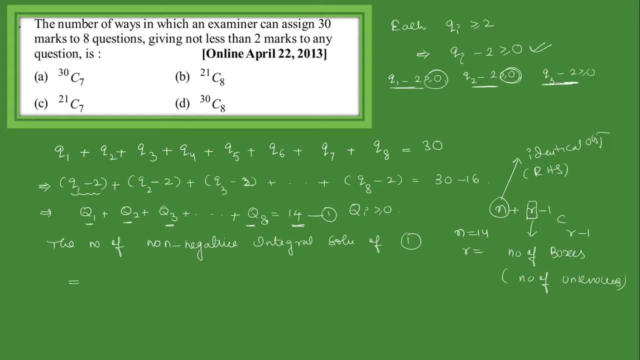 Number of variables or number of boxes. How many boxes? q1,, q2, q3, up to so on q8.. So r is equal to 8.. Apply the formula 14 plus 8 minus 1, c, 8 minus 1,. 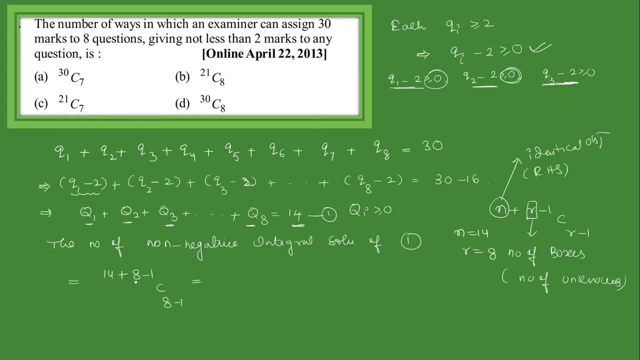 which is 14 plus 8, is how much? 22.. Yes or no? 14 plus 8 is 8.. 22 minus 1 is 21.. And that is c 9. So 21c, sorry, sorry. 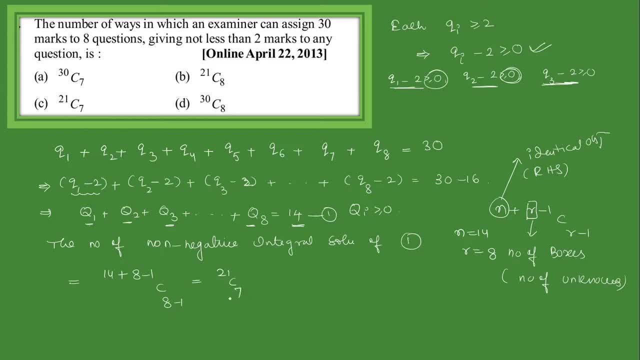 a small mistake: 8 minus 1, 8 minus 1 is 7.. So 21c1.. You can see 21c7,. sorry, 21c7. you can see in the c option. Okay, So this question you can see. 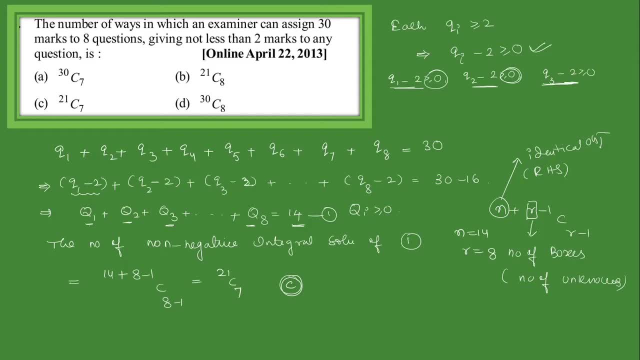 a practical question given to you, but we converted this into the equation Right So you can use this linear equations whenever such type of questions given to you. Let's see one more question so that you will understand better. Now, here you see. 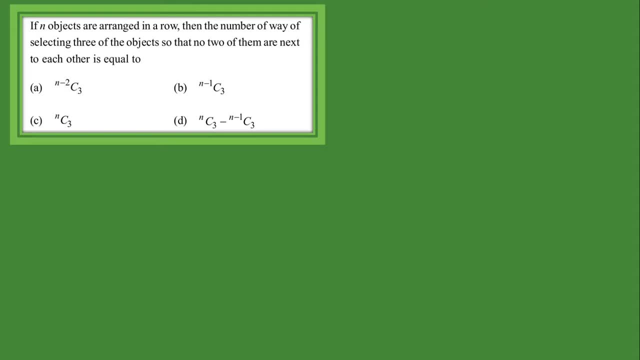 if n objects are arranged in a row, then number of ways of selecting three of the objects so that no two of them are next to each other? No two of them are next to each other, So how many objects are arranged in a row? 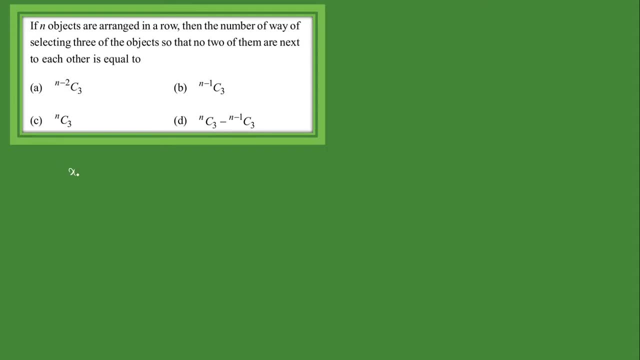 N objects. Let's say, here you have an object x1,, you have an object x2, you have another object, x3, x4, like this, You have n objects arranged in a row. Now, from this, you have to. 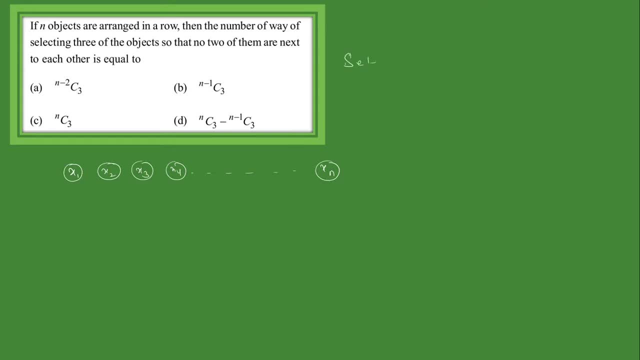 select. how many objects We have to select? we have to select three objects, Any three objects you have to select, But these three objects, no two of them, are next to each other. So means, for example, in this, for example: 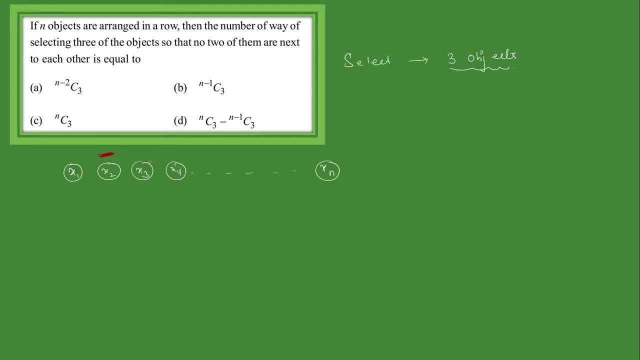 if I take x2 object, the next object is not x3. Because of he says that condition, No two of them are next to each other. So after selecting x2, you cannot select x3.. If you want, you can select x4,. 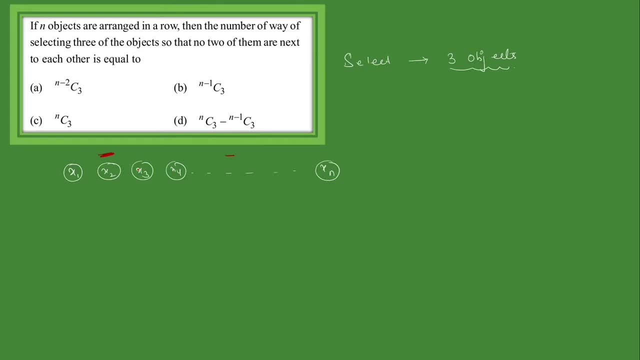 or, if you want, you can select x5,, or, if you want, you can select x6, but not x3.. What is the meaning of this? In between any two selections, in between any two selections, there must be one object between them. 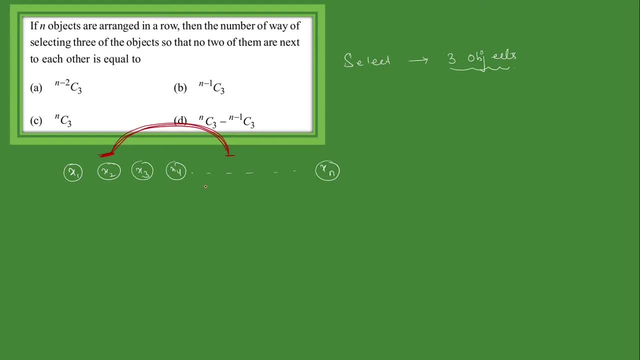 At least one object should be there between them. They are not next to each other. I hope you understood this. What is that? In between two selections, in between two objects, there must be at least at least one object should be there. 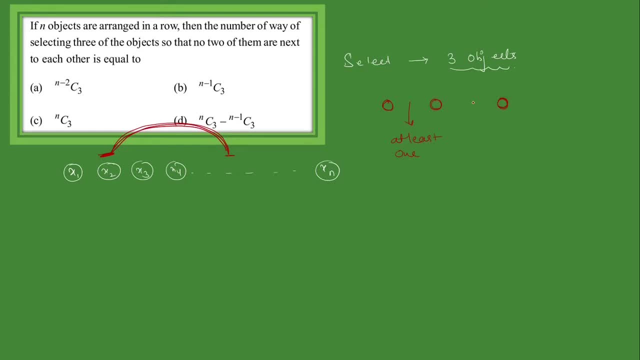 And after the second, whenever you select the third one, at least one object should be there again in between second and third. At least one object, Right? So this is actually the idea of the problem. Let us say I selected one object here. 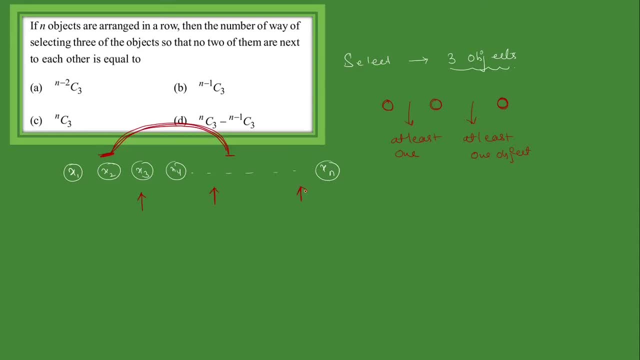 second object I selected somewhere and third object I selected somewhere. Now, Now, how many objects are there between- sorry, before- the first object? whatever we selected, the first one before that, how many objects are there? Let us say, that is something y1.. 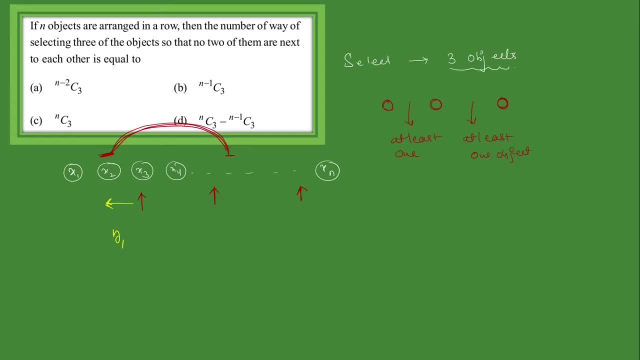 Number of objects: Number of objects before, before the object selected, the first object selected. Next, y2 is number of objects between the first object and second object, And y3, the number of objects between second object and third object. After selecting the three. 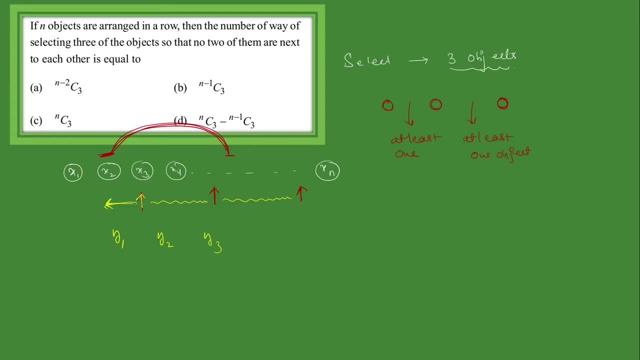 objects. I am supposing that before one. for example, if you selected x3, how many objects are before x3? Two objects, That is your y1. So here y1 is equal to 2.. For example, I am telling you: 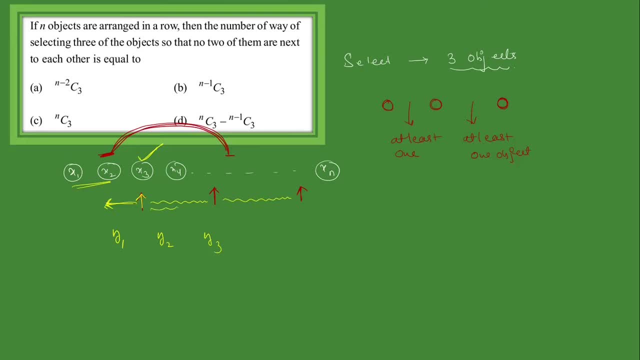 And in between first and second, how many objects are there? I am supposing y2.. In between second and third, how many objects are there? I am supposing y3.. After the third object, whatever the object left with us. 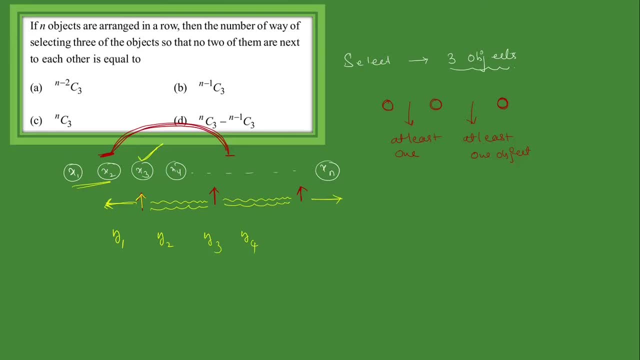 we will suppose as y4.. Then can you tell me what is y1 plus y2 plus y3 plus y4? is going to be y1 plus y2 plus y3 plus y4 plus y4. value going to be what? 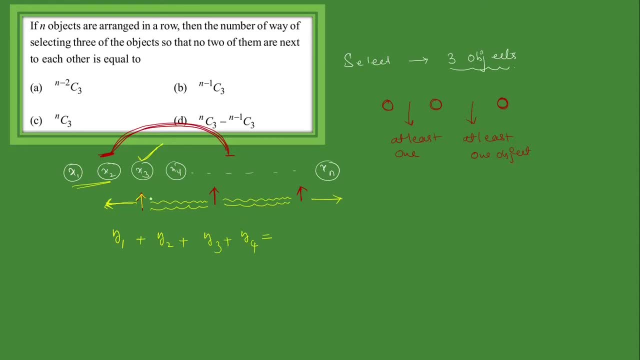 Can you tell me that, Because of see how many objects in a row, you selected three objects, So, other than three objects, everything is counted in this Yes or no Before first object, how many are there In between first and second? 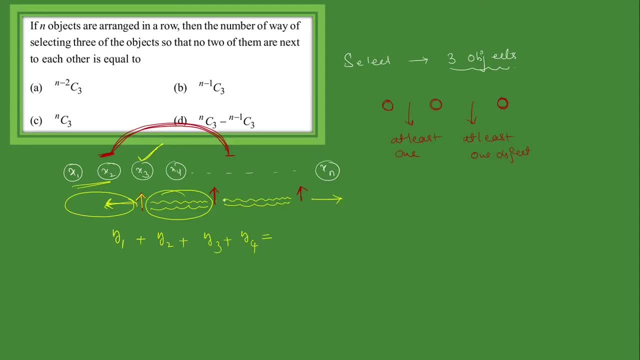 how many objects are there In between second and third object? how many are there After third? how many objects are there? So how many objects you are leaving in your counting? These three objects you are leaving Remaining, all objects are counted. 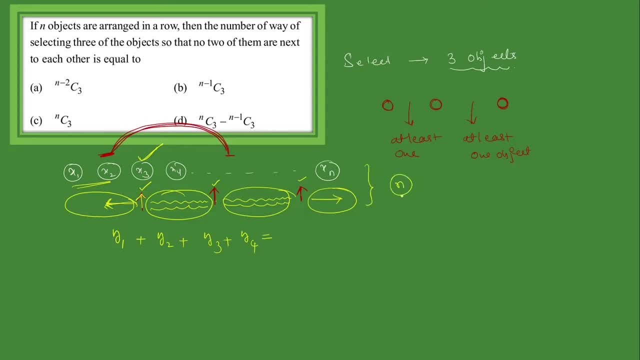 So total number of objects are n. Total number of objects are n. In your counting only three objects are missing, which we selected, So n minus 3.. So y1 plus y2 plus y3 plus y4 should be equal to: 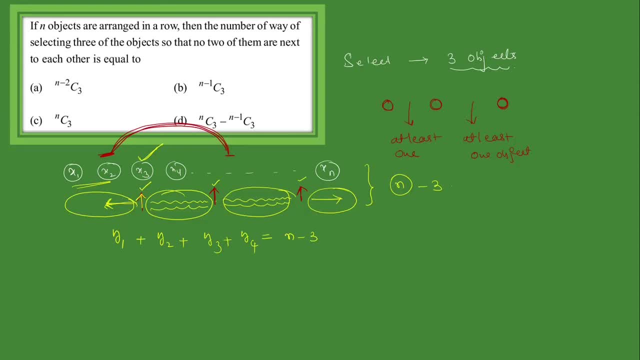 n minus 3.. Now, in between first object and second object, at least one object should be there, Otherwise they will become consecutive, They will become next to each other objects. So there is at least one object in between first and second. So in between first, 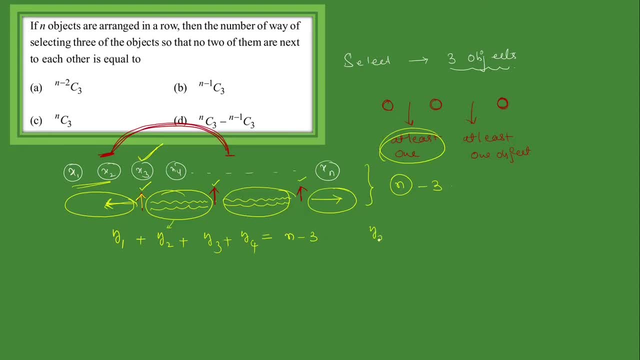 and second. what is the number? we supposed y2.. So y2 should be at least one, Means y2 greater than or equal to 1.. Similarly, in between second and third, also in between second and third also, there should be at least what? 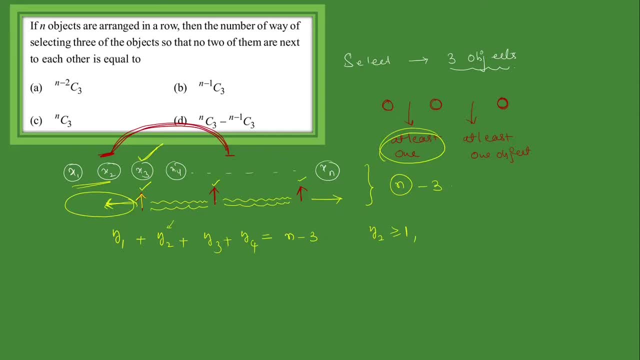 One object should be there. In between second and third object, at least one object should be there. What is that? y3.. So y3 should be greater than or equal to 1.. And what about y1 and y2?? 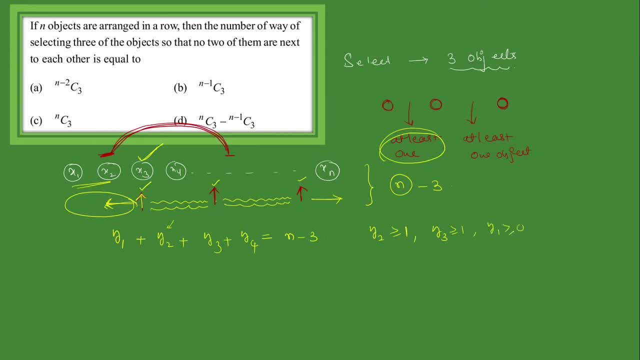 There are no conditions on y1 and y4. So y1 should be greater than or equal to 0.. y4 should be greater than or equal to 0. But if you want to apply the rule that non-negative or positive integral solutions. 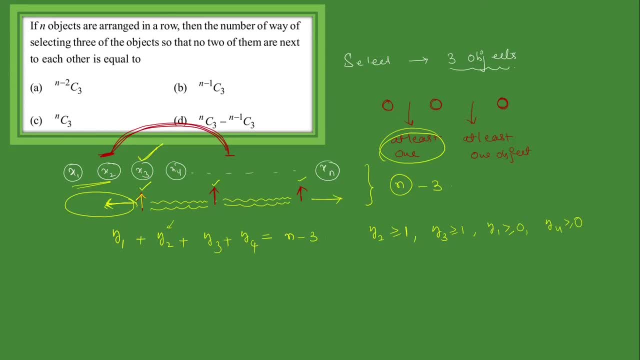 whatever we derive to 2 formulae: Non-negative, non-negative nature. Here y1 is already non-negative. There is no problem with this. y4 is already non-negative. But you can see here y2 minus y2 is not non-negative. 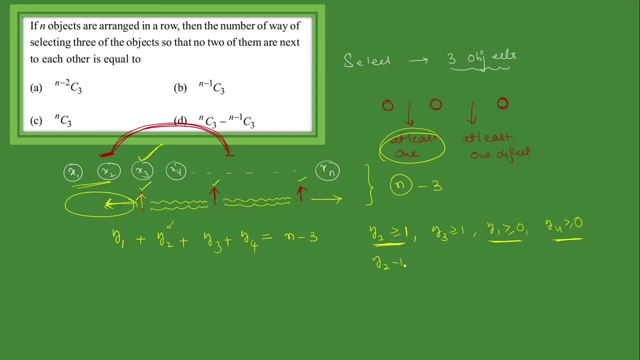 It is 1 or more than 1.. So to y2 minus 1 is greater than or equal to 0, and here y3 minus 1 is greater than or equal to 0. So we are going to convert this y2 and y3 from the equation. So y1 plus y2, I will write y2. 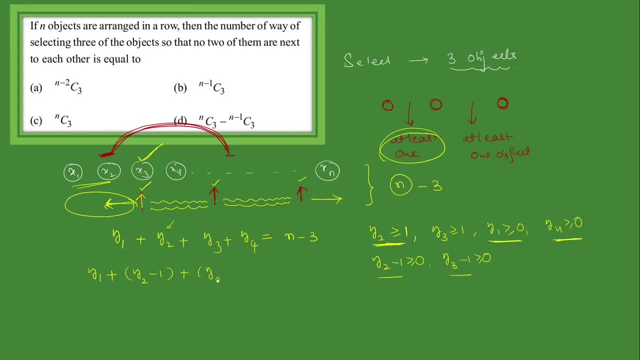 minus 1 and y3, I will write y3 minus 1 and this is y4 is equal to: because of you subtracted 2 from the left hand side, you have to subtract 2 from the right hand side also, So n minus 3.